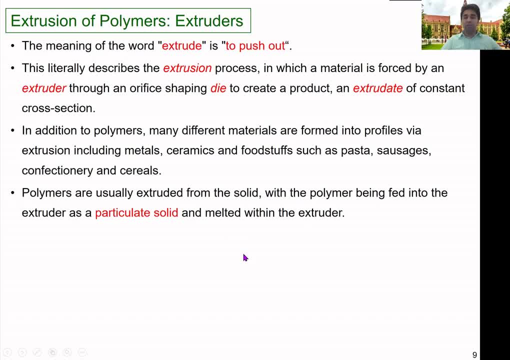 with the polymer being fed into extruder as a particulate solid- it could be the powder form or pellet or the the granule form- and then that material is melted within the extruder and then after that push it out to the die to get into the desired shape. As we discussed already, the normal in polymer. 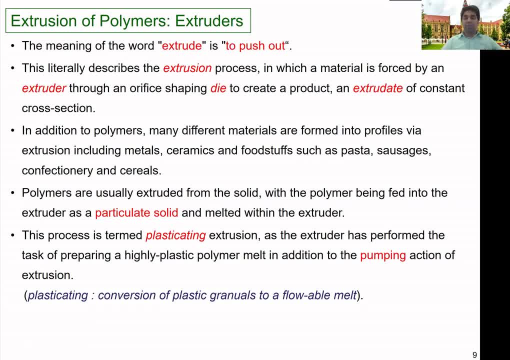 processing. we just feed the solid material into the machine and then, after that, it becomes molten and then we can push it into a die. Okay, so the? therefore this process is termed plasticating extrusion. So what is the meaning of plasticating is, that is, the conversion of plastic granules to a 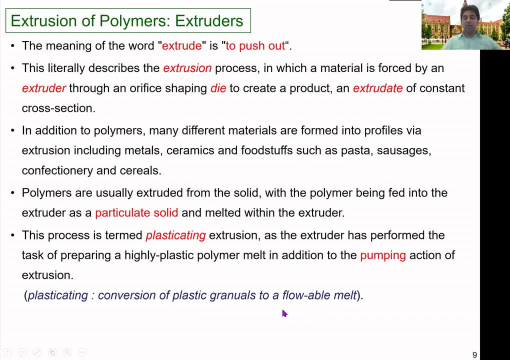 flowable melt- Right, it was the plastic materials which were in solid form, and then converting it into a flowable melt is known as the plastication process. Okay, so normally in extruders, melt is plasticating, and then that melt can be used to form different shapes as we need In industry. 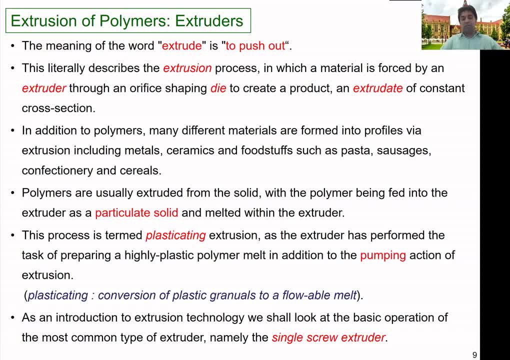 there are a number of different type of extruders. Of these type of extruders, single extrude extruder is the most commonly used type, so therefore I'm going to concentrate on single extrusion extrusion. actually, As I mentioned before, now you can see the classification of extruders into different 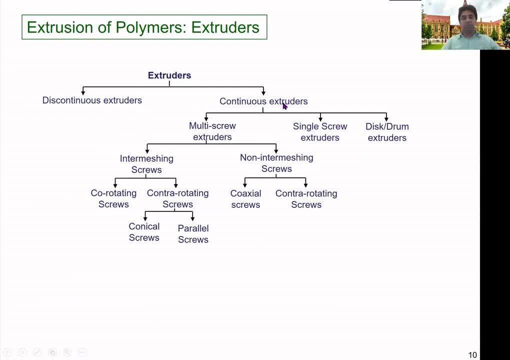 types. So this: continuous extruders- continuous extruders- okay, and then you could see the continuous extruders again. you can just break that into three different categories. multi-screw: it could be more than one screw. single extruders: okay. that is the most commonly used machine in. 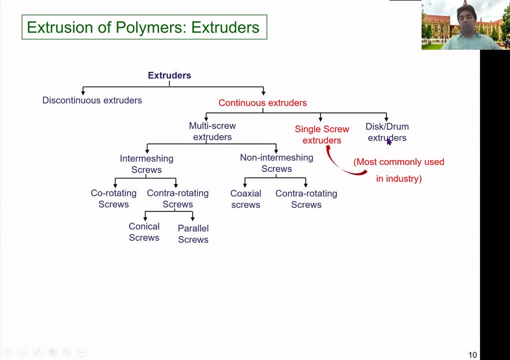 the plastic processing industry and this dicks and drum extruders- okay, that is another type. actually, Look at the multi-square extruders. we can classify that into two different categories as intermission screws or non-intermission screws, or and likewise, so there could be several other. 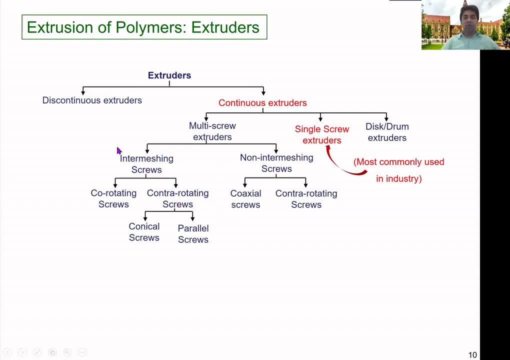 categories. uh, we can classify those extruders into Right. so let's look at what is the main difference between continuous and discontinuous extruders. The continuous means actually utilize in a rotating member such as a screw- okay, and achieves a continuous output of materials. 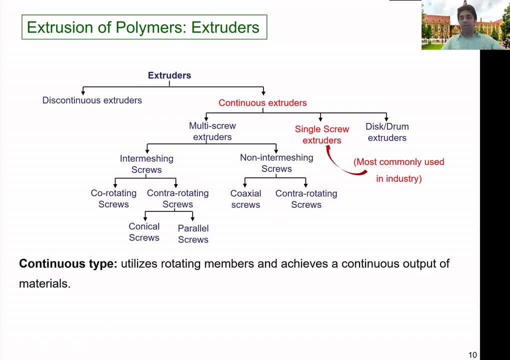 If you can provide the material continuously, that means the solid material, into the machine continuously, so then you can have a continuous output. so that is the idea. okay, so then output is continuous as long as you feed the material into the machine. okay, then. the discontinuous type is bit different. it's like a reciprocating motion. 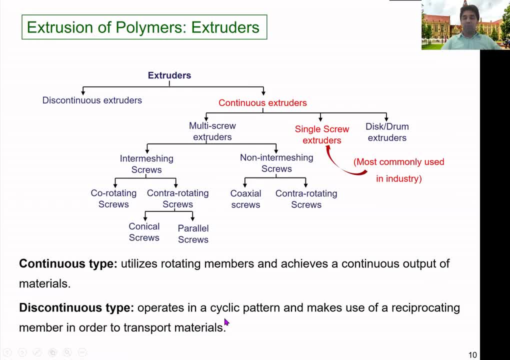 okay, those type of extruders operates in a cyclic pattern and makes use of the reciprocating member in order to transport materials. okay, like injection molding. so they produce some certain amount of melt. we call short size, for example. so then, once the desired amount of melt is being just formed or created within the machine, so that 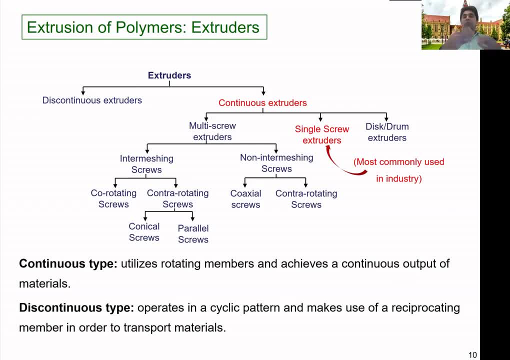 amount will be just pushed into a die or just pushed out of the machine by a reciprocating member, so they, then we can use it, so this can happen like a continuous cycle. so it has been pushed and then again the the member goes back and then the next shot will be ready when we need. 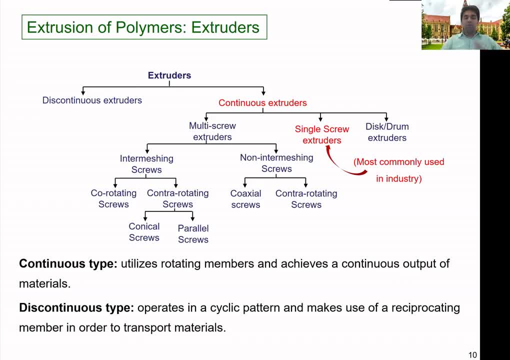 to have the next shot, to produce the next product. okay, so you can understand now the difference between the. the continuous type means we can provide output continuously, but for the discontinuous type, that we can control, it will provide the material time to time or with some certain the frequency as we just set it up. so 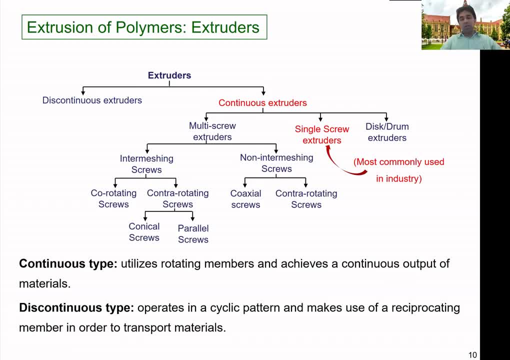 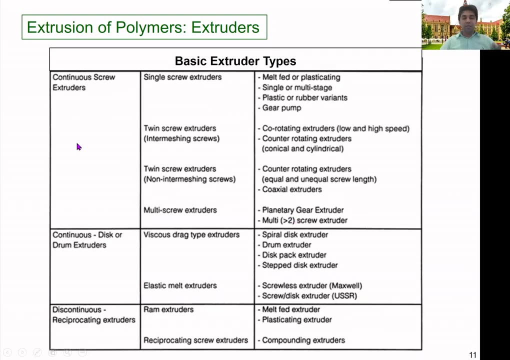 kind of good example would be the, the injection molding machine. it has a reciprocating screw and also it has the rotary motion as well. okay, so here i'm going to just look at the single extruders used in polymer processing. here you can see some extra information relating to some sort of basic: the extruder types, the. 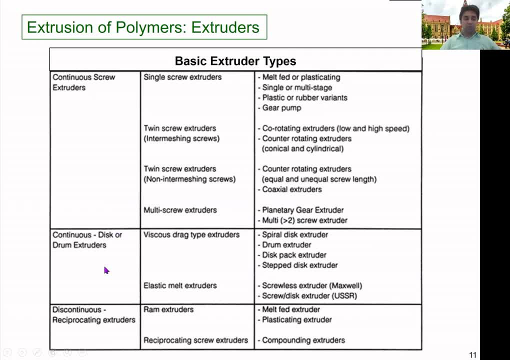 continuous two extruders, the continuous dicks or dumb extruders, the discontinuous reciprocating extruders. right, so you could just read through this and then here you could see some other important information relating to those type of extruders. so now i'm going to look at the specific 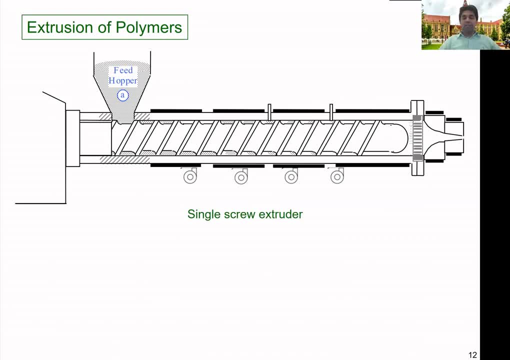 components of a single extruder. here you can see the arrangement of a single extruder. so i'm going to explain the part by which we are going to explain the part by which we are going to explain part. so then you can understand, uh, their function and why they are important actually. so here you. 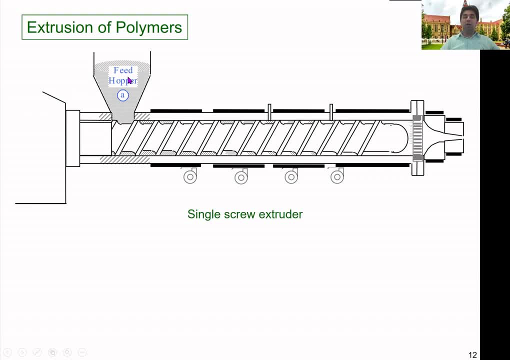 can see the feed hopper. so this is the place that we just call uh, the feed in the material, into the machine. okay, so you can see that it's the gravity feed. actually, once you just fill the material into this hopper, so it will just the force into the, into the, the chamber, or, in this case, into the. 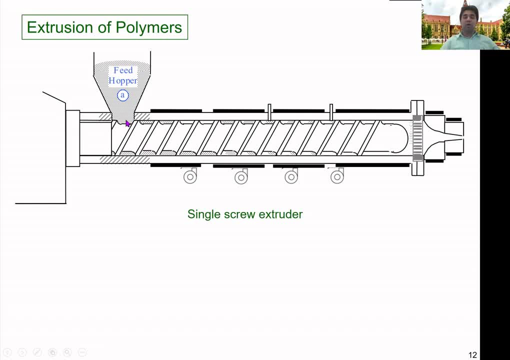 barrel, uh, through the gravity, okay. so there could be some kind of force feeders as well, so you can just they push the material, okay, and then we can control the feed rate. but here it's completely depend on the gravity. so then, as material is just being taken out from the machine, from here, 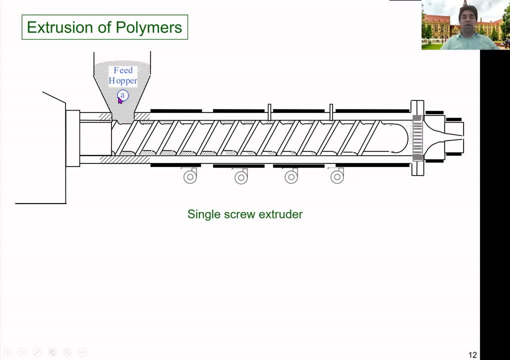 so then the the new material will be pushed in or dragged into the machine. uh, from this point? okay, hope it is clear, right. so then, uh, the. this is what we call the feed throat. okay, though, that feed throat is really important again, so sometimes we can just control the temperature in the feed. 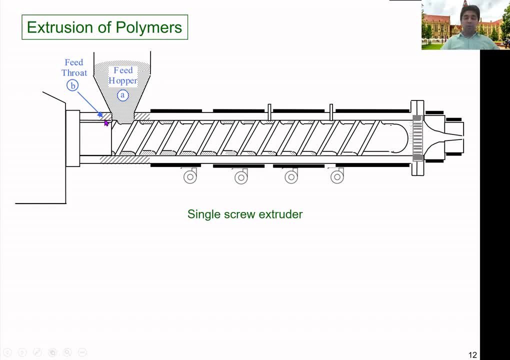 throat, okay, or we can cool it down as well. so we don't want any material to be molten at this point. okay, so we want to have them in the solid state, so then they can convey easily along the screw, right? so therefore, in some the extruders. 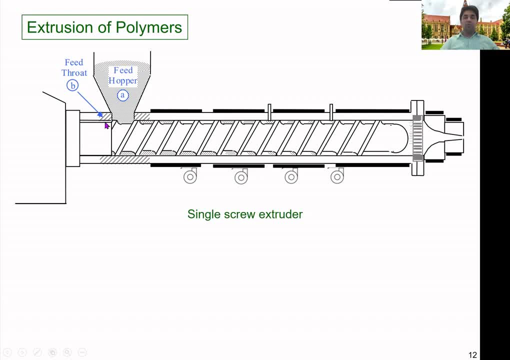 there could be the feed throat cooling as well. right, so we have to maintain the temperature to make sure that proper conveying takes place across the along the screw. actually. so this is the extruder barrel. actually so it's. it has a certain thickness, so the thickness of this barrel could be two, three. 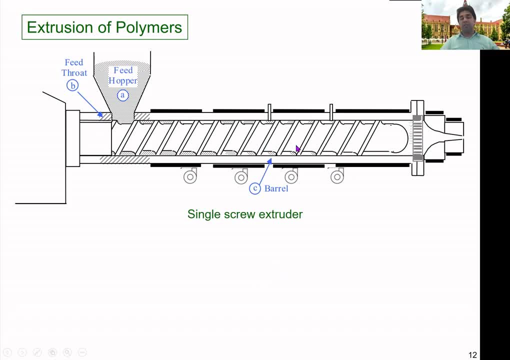 centimeters sometimes okay. so there could be a pressure generation inside the machine while it has been working. so the pressure could be 50, 60 bars or even higher, depending on the size of the extruder. so therefore we have to have the barrel that can support that certain amount of pressure. 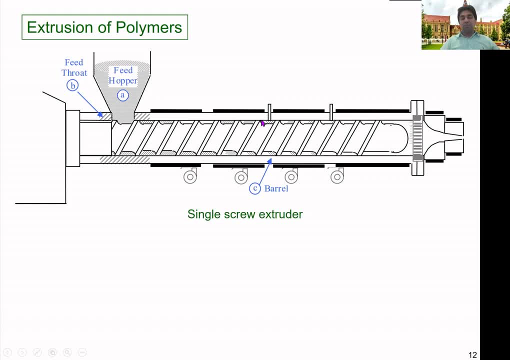 okay, and this is a smooth barrel surface. but there could be some new extruders. comes with some glued barrel as well to promote the melting and the conveying of the material. so here we have the electrical resistance, the band heater, so if it is a the circular barrel, so then we can have some cartilage heaters that we can wrap around. 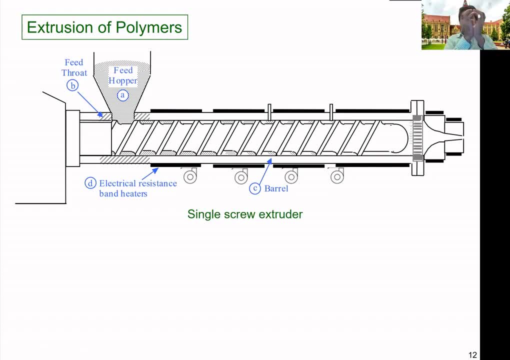 wrap around the barrel. okay, so we can open it like this and then place it and then close it or clamp it. so we we call them cartilage heaters, so then we can wrap them around the barrel depending on the length of the extruder, so there could be a number of different heater. 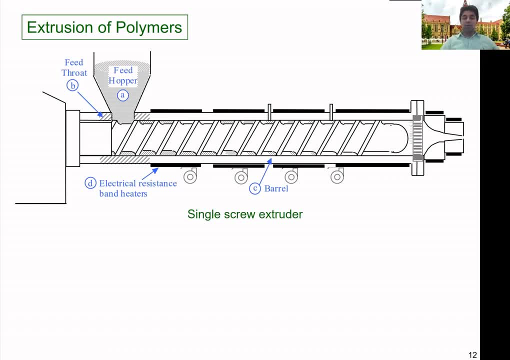 bands or the heating zones along the extruder barrel. okay, so the heaters could be within along the barrel, or it could be within the, the dies or in the other units as well, as we have a number of different heaters, so we have to maintain the temperature profile in axial direction. 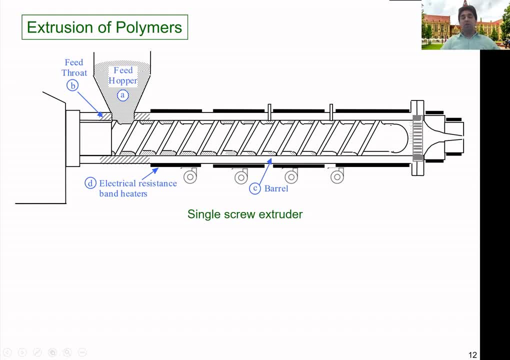 to to ensure the proper conveying of the material or the proper melting of the material. so this is the screw. that is the main component of the machine. actually, it has a function of conveying the material and also converting the material from solid state to the molten state while it has been conveyed along the screw. right, the screw is having a normally 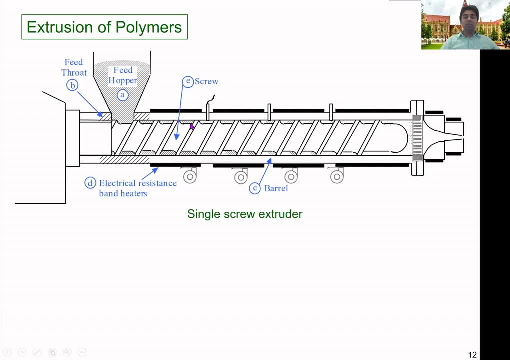 uh, specific, uh the design. so normally in this, in this zone, we call it the feed zone. uh, you could see these grooves or the channel depths are high. okay, so then channel depth is gradually decreasing as it is going through this direction. okay, that is what it normally happens. i'm going to show you. 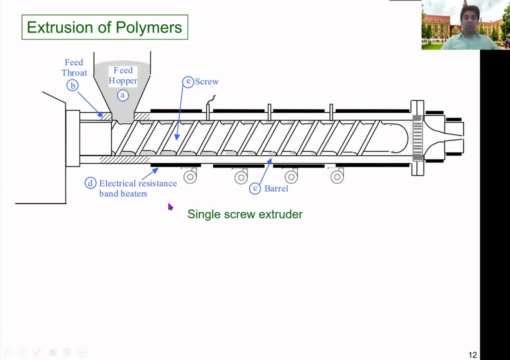 some real screws using industrial applications in incoming slides. actually, here it's the dry. dry means the unit that we use to rotate or return this group. so it it could be a dc motor or ac motor. it could be a hydraulic drive. so the most commonly used wars for small extruders is the. direct current motors, but nowadays they do notante. that is the unit we use to rotate the turn this screw. so it could be a dc motor or ac motor, it could be hydraulic drive. so the most commonly used was for small extruders- is the direct current motors. but nowadays the extruders are used to perform high current relation with high activities. 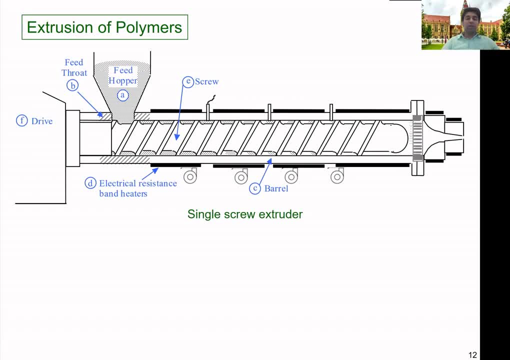 It could be AC motors or the vector controlled. AC motor drives could be used with some extruders. OK, so normally that could be a gearbox between the screw and the drive, But in new extruders comes with a direct drive as well. 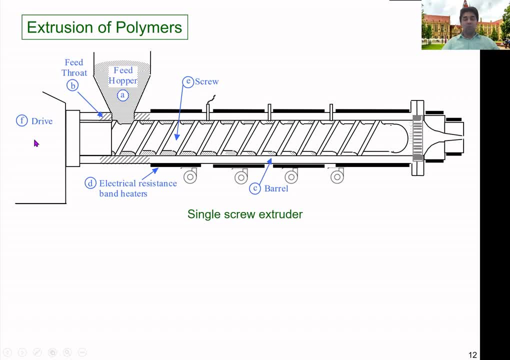 That means that the motor shaft is directly connected to the screw, but it is not that common, So most of the time that could be a transmission or the gearbox between the motor and the screw. Yeah, so we have to use the thrust bearing if you have the transmission unit. 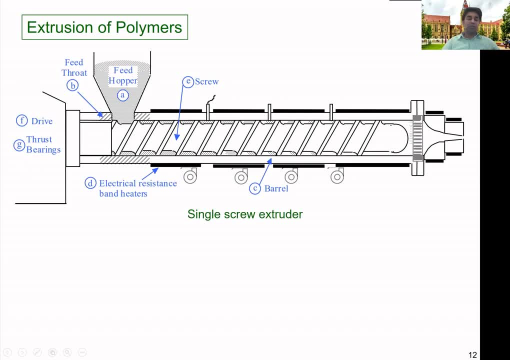 So then we can smoothly transmit the rotation between the drive and the motor. Right, So then the breaker plate actually. So here you can understand that as the molten material comes along this way now, So while the squeeze beam is there, it will be rotating, So then it has a swirl motion. 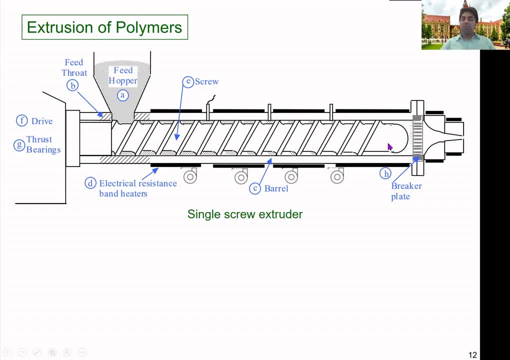 OK, so it has a rotating motion or swirl motion at this position, But we need to have a linear flow of material that is coming out of the barrel. OK, so therefore, the breaker plate can be used to convert the rotary motion of the melt into a linear motion. 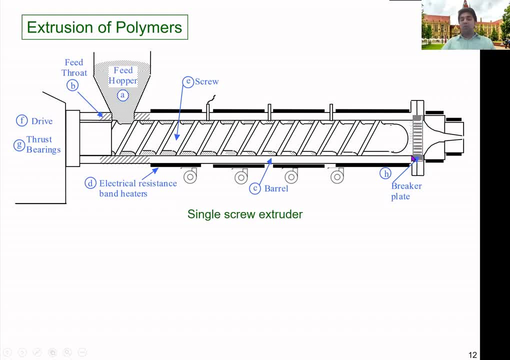 OK, And also, as we place this, it could cause to create some extra pressure at this position as well. Of course, it is just blocking the flow. It has only small holes, So therefore that would increase the pressure Inside the chamber as well. And then the screen packs are also being used. 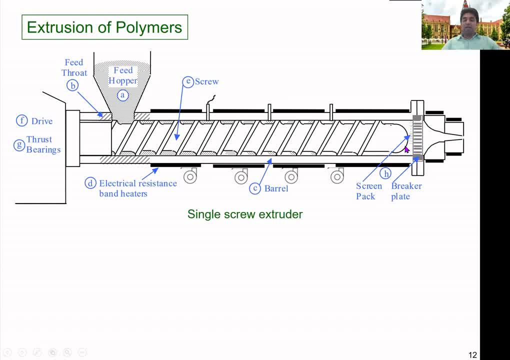 So before the breaker plate we use something called a screen pack. So that is mostly to just purify the molten material. If there are impurities or unmelted particles, the screen pack stops them without being pushed into the die. actually, 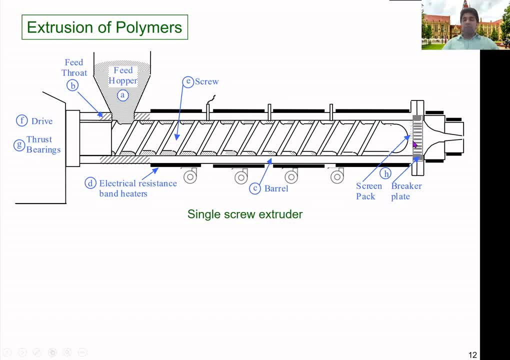 Here. we don't want any unmelted particles or any impurities to come out of the machine. So therefore, the screen pack is just there to just make sure that, to stop those type of unnecessary materials or undesired materials. OK, so again, this will create some extra pressure because it is being placed here and trying to block the flow. 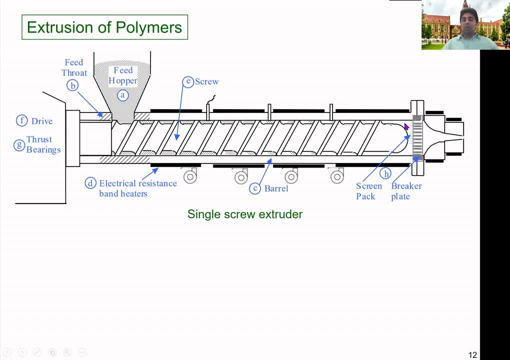 And also trying to control the flow here. OK, sometimes this screen pack should be changed time to time. It could just create some blockages of the material as the accumulation of the material on top of that. So therefore we have to replace the screen pack or clean it up time to time to maintain the proportion. 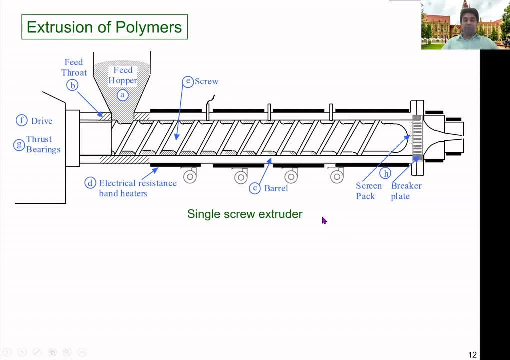 OK. So therefore, we have to replace the screen pack or clean it up time to time to maintain the proportion In comparison to operational conditions. and then this is the die. So die is the unit which forms the material into the desired shape. Within the die, there is a cavity. The cavity is the shape of the product that we need to manufacture using the molten polymer. 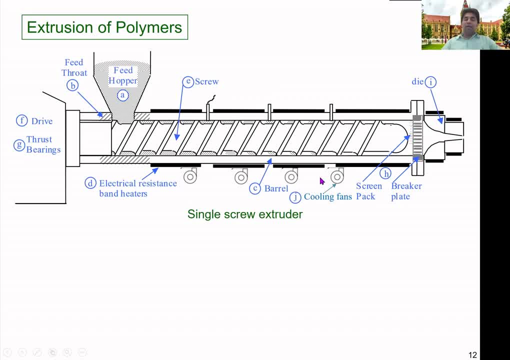 So then cooling fan is here, So here we have to maintain the temperature actually. So if you discuss about the axial temperature profile, normally what we do is that: so we have the lowest temperature in this zone, So in here we have the normally solid material. 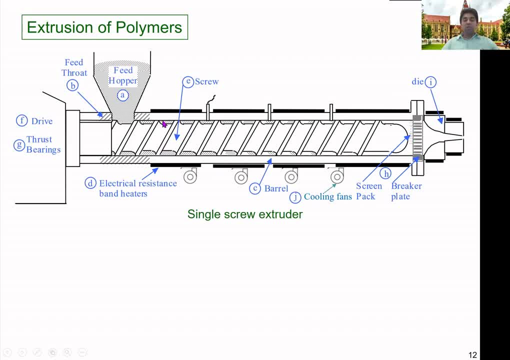 normally solid materials. so we don't want early melting of the solid material. so then we normally set a low temperature in this region, okay, so for example it's 150, 170, 200 and 220. okay, so that will ensure the proper, uh, the conveying of the material. so that means it will just make sure that proper. 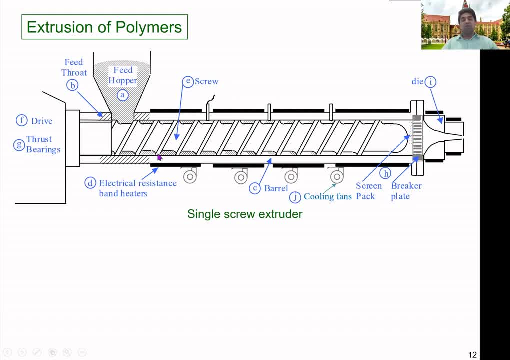 the frictional heat generation and viscosity dissipation as well during this zone. okay, therefore, the selection of the set temperature is also important during the process. okay so, but we want to maintain the barrel temperature, so therefore, uh, there could be cooling pans. okay, this might not work continuously, but let's say we set the temperature to be like the 200 degrees at. 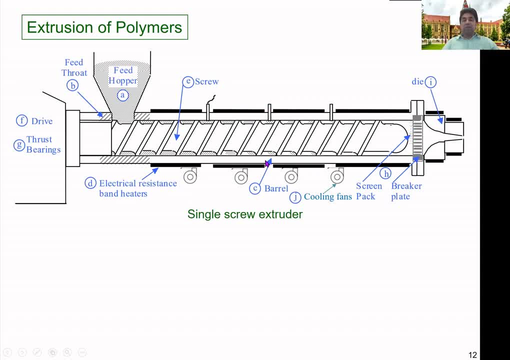 some place, or 170 degrees at here. so then if it is just exceeding that value, this cooling pans will automatically turn on and then try to maintain the temperature. actually, here there are something called pid controllers to look at the temperature if the temperature of these heater bands going. 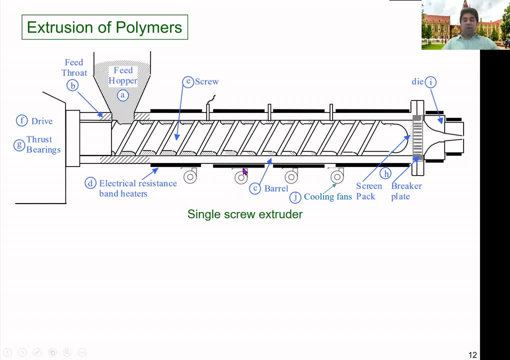 beyond the set value. so this is could just known. actually, one of the issue is that so we have set this temperature to be 170, but there could be some internal heat generation as well. so therefore we have mainly three main modes of heat mechanisms: the, the conductive heat through this uh, the heaters, and also frictional. 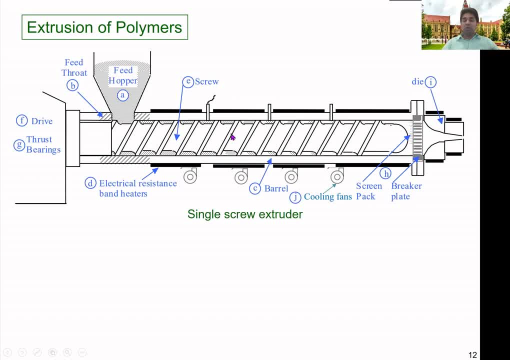 and viscosity dissipation inside the barrel. so therefore we don't know. actually, the temperature is going to be the same value as we set outside the barrel. okay, for some reason, if the temperature is going beyond the set value due to the the extra addition of the heat inside the machine, 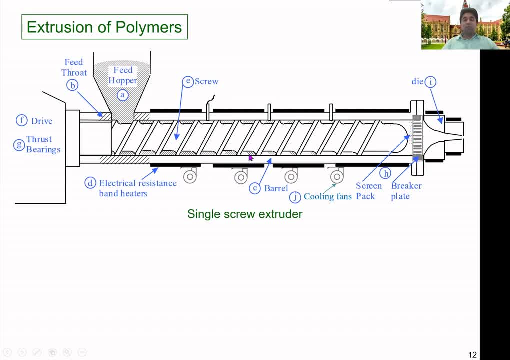 so the- these are the- the cooling pans can turn on and then cool it down to the desired value again. then the process monitoring is also really important aspects. we can use some thermocouples, pressure sensors in different locations to observe the temperature and pressure of the of the of the process. so, as i mentioned before, the screw is the main component of the. 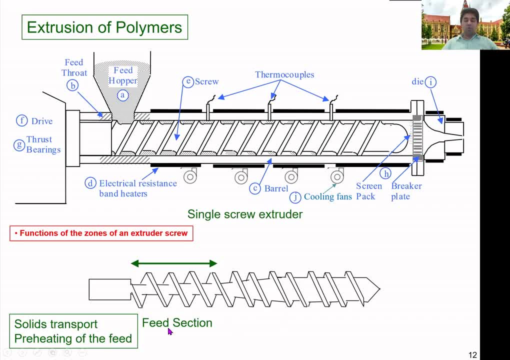 machine. it has three main functional or geometrical zones. okay, the first zone i mentioned you, that is the solids conveyed or the feed section. so you can see that here the channel depth is reasonably higher compared to the uh, the, the melting zone or the melt conveying zone. and then the second, after the solids conveyed, or feed section. 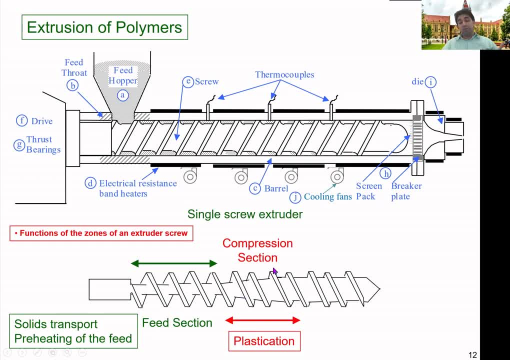 so we'll have the compression section or the plastication section or others equal. it's melting section. so here you could see that the channel depth is gradually the decreasing, or it is just trying to get the smaller clearance between the barrel and the screw surface here. so then the final. 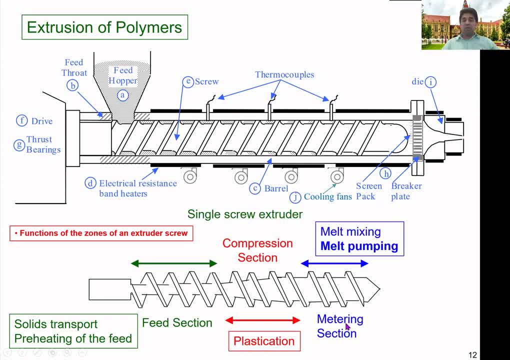 we have the melt mixing or melt pumping section, or sometimes we call it the metering section. in this zone we have the shallowest channel depth. okay, it's, it's over. here we cannot just indicate some exact the, the boundaries for these the zones, but they are really indicative. the the first feed. 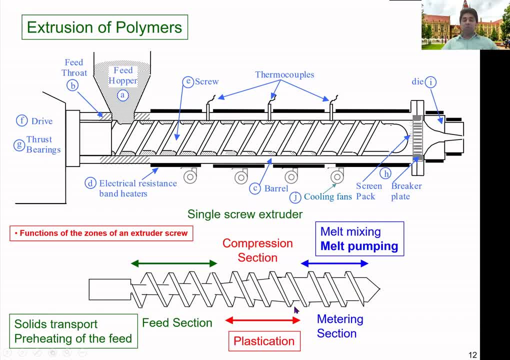 zone, the compression zone, and the, the mixing zone. ideally, in the, in the feed section, material should stay, uh, the solid, while absorbing the heat and then melting should start at this point and then, as the material reach into this position, so they should be fully molten. so then, finally, those. 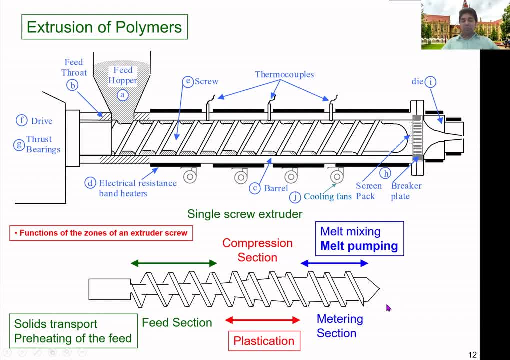 material can mix and then we can pump them out from the machine. actually, actually, the screw is trying to control all of those actions and there are a number of different type of screw geometries are used in industry. so, depending on the type of the material, sometimes you have to. 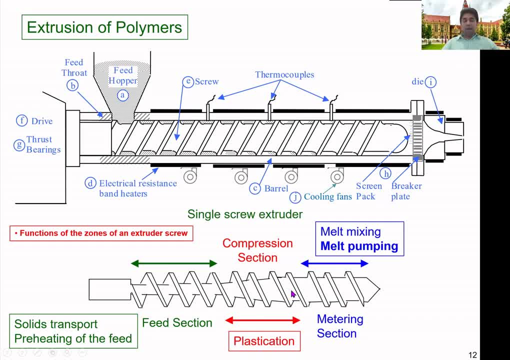 just select the suitable. uh, the type of screw and also screws could be in different arrangements. this is the really most common and conventional type used in industrial applications, but nowadays there are some new screw designs, like barrier plated screws, so they have a different arrangement of these, the channels or the grooves. okay, so i can show you some of them in the coming slides. 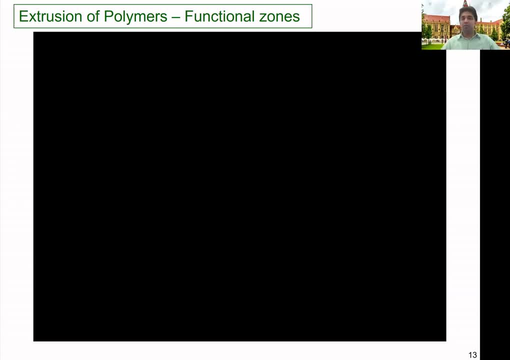 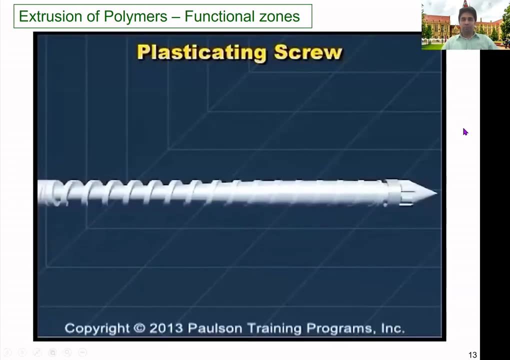 this video provides a nice explanation on the functional zones of an extruder. the simplest screw design has three zones: the feed zone, the compression or transition zone and the metering zone. the feed zone has the deepest flight depth, allowing the greatest volume of granules to fall. 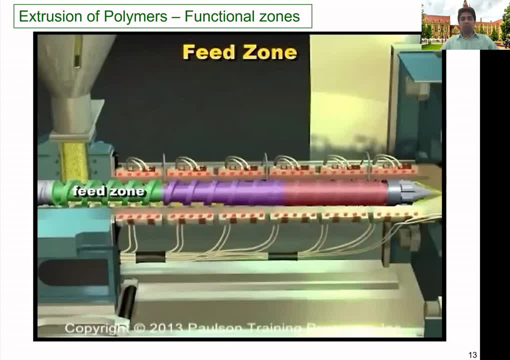 into this zone. it's where plastic melting begins. next is the compression or transition zone. this zone has gradually decreasing flight depth. the compression zone is where melting of the plastic pellets should be completed. the feed zone has the deepest flight depth. the last zone is the metering zone. it has the least flight depth. 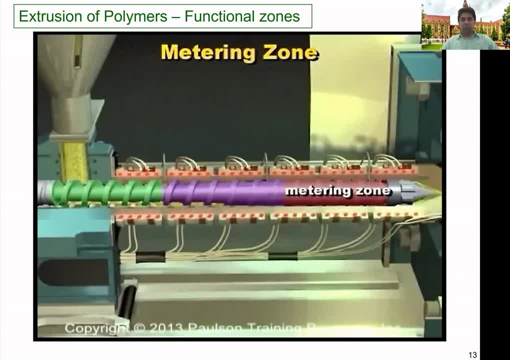 and so is the most restrictive to flow in this zone. the plastic should be thoroughly mixed and should be at a uniform temperature. the ratio of the flight depth in the feed zone to the flight depth in the metering zone is called the compression ratio. the compression ratio affects: 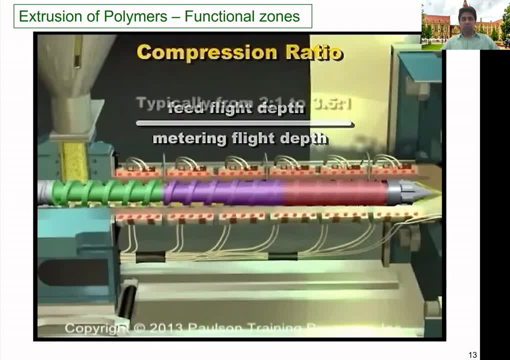 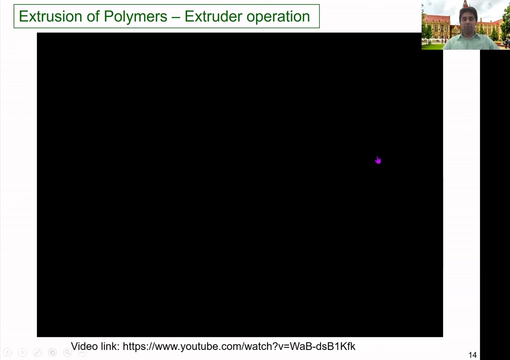 the melting ability and the output of the screw. typical compression ratios for thermoplastic screw designs are from 2 to 1 to 3 and 1 half to 1. thermoset injection molding screws have little or no compression ratio, and also this video provides a nice explanation on the extrude operation as well. 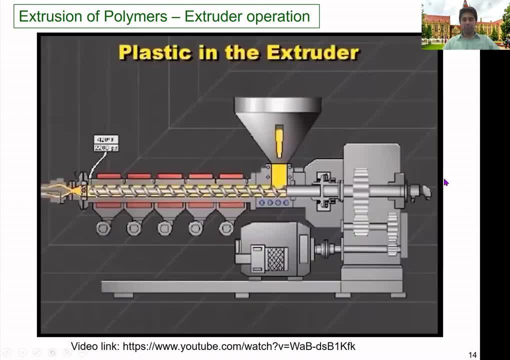 now let's look at the end form and, too, used them well indeed, at the inside of an extruder to see how it works. The plastic raw material in this hopper travels by gravity to the feed throat and drops onto the rotating screw. The rotation of the screw. 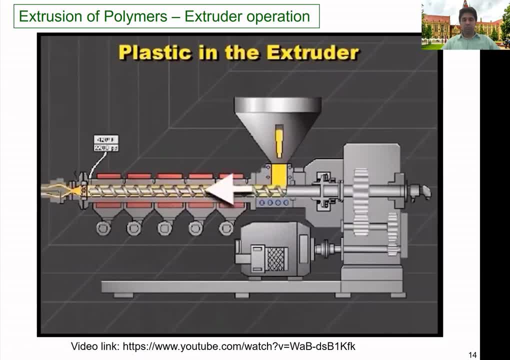 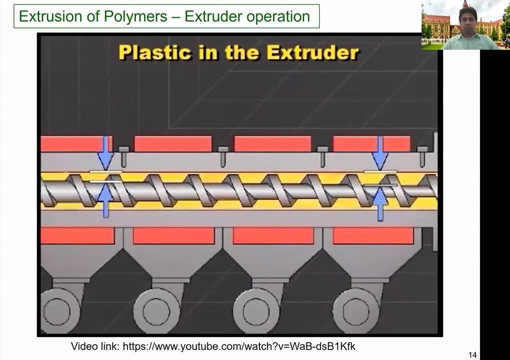 conveys the plastic forward through the heated barrel. As the plastic is conveyed forward along the screw, the channel depth decreases, forcing the plastic through a smaller area. The combination of compression and screw rotation causes friction, which generates heat. This is called shear heating. 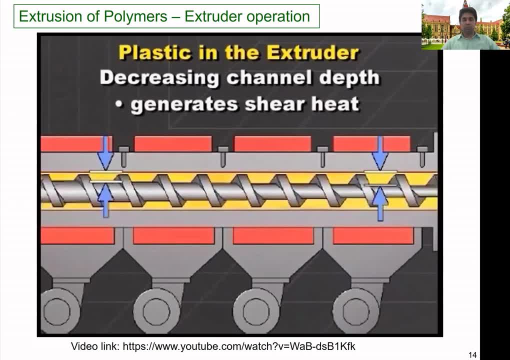 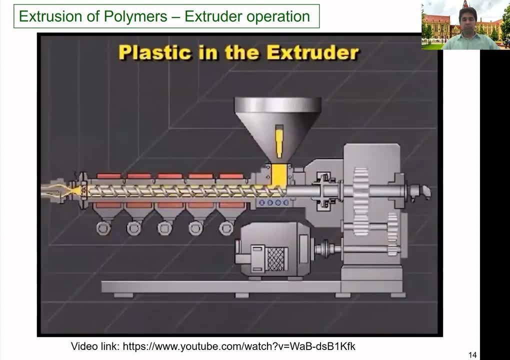 This heat, along with the heat from the barrel heating system, melts the plastic. By the time the plastic is conveyed to the end of the screw, it should be well mixed and at a proper temperature and pressure needed by the die. The plastic is called a melt at this stage. 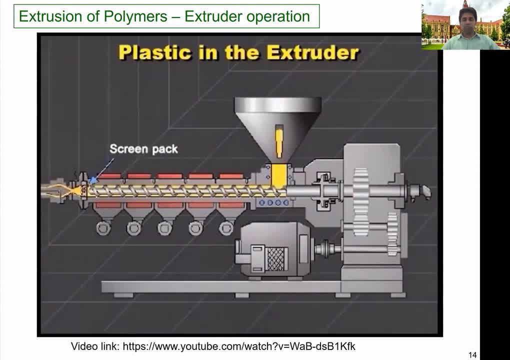 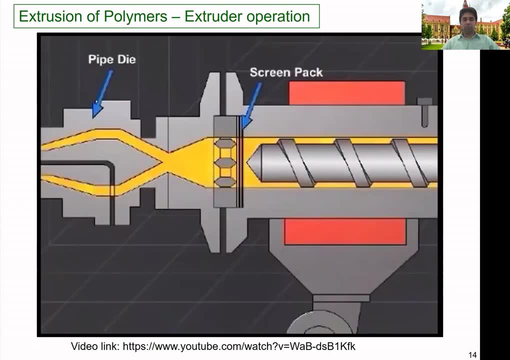 Beyond the screw there can be a screen pack. The screen pack is a set of wire mesh filters that the plastic must flow through. The screens are typically from 20 to 100 mesh, which indicates the wires per inch. The screen pack is supported by a breaker plate, which is a sturdy metal plate. 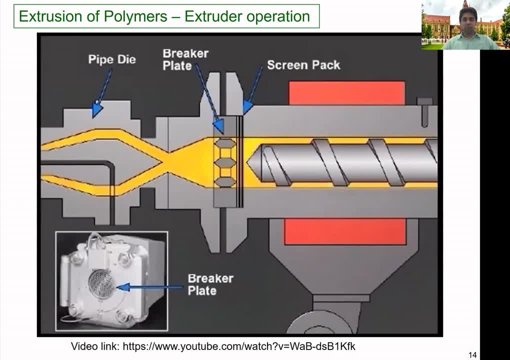 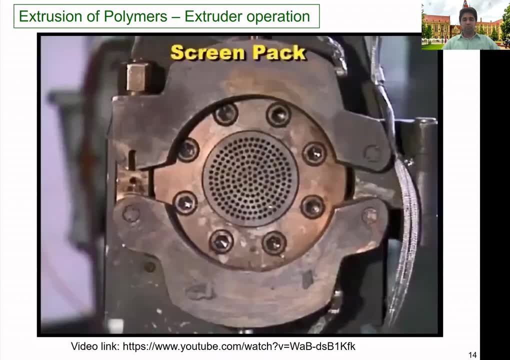 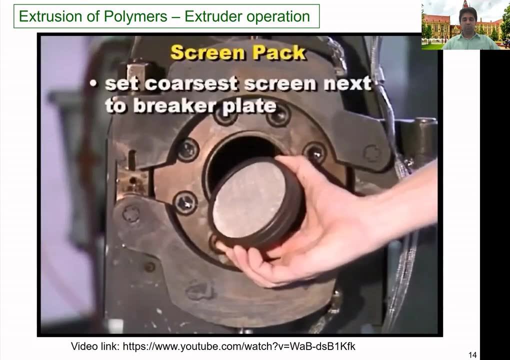 with many holes for the plastic to pass through. The screen pack filters contaminants from the melt. The screen pack must be set in place with a coarsest screen next to the breaker plate so each screen can support a finer one. Otherwise the pressure difference may break the fine wires. 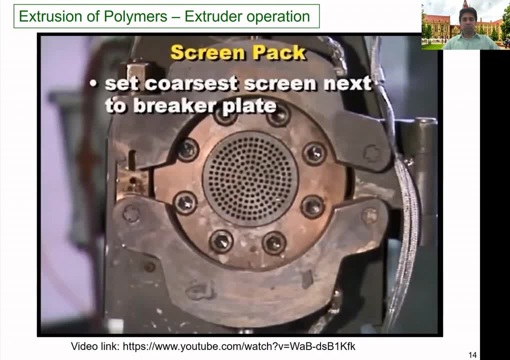 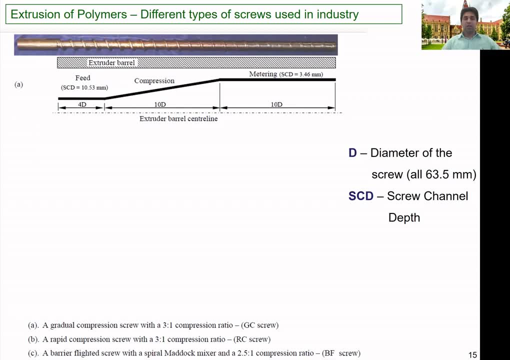 contaminating the product and possibly doing permanent damage to the die. Here you can see that some of the common screw designs used in current industry actually. So this is what we call a gradual compression screw. Here you could see that the D indicates the diameter of the screw actually. So all of these screws are 63.5 mm in diameter. 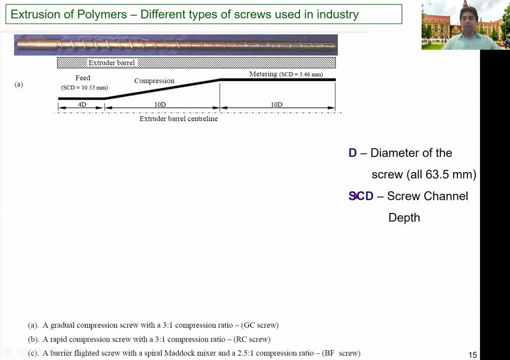 Right, And also the SCD refers to screw channel depth. Okay, So if you just remember that in the previous video they discuss about the channel depth, here In the peat zone, the channel depth you could see that is 10.53 mm for this screw. 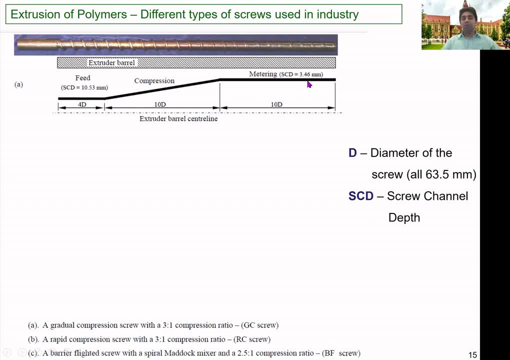 And then in the metering zone it is 3.46 mm only, So you can clearly see that the channel depth in the metering zone is the lowest compared to the peat zone. actually, Okay, The channel depth in the compression zone also gradually decreases as well, Right, 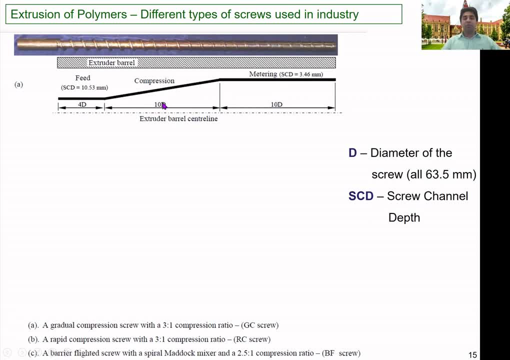 So here the D indicates the diameter. So you could see that the length of each zone, here the peat zone or solids conveyance zone, and then compression zone, and here the metering zone Right The peat zone, is four times of diameter in length. 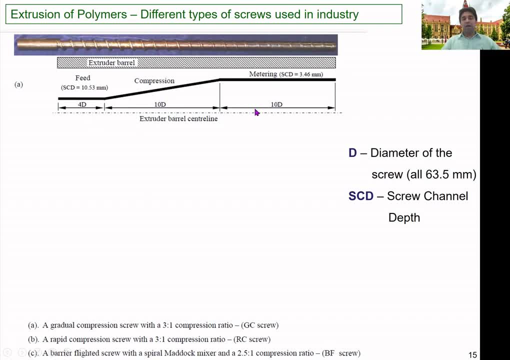 And then the compression zone is 10 D in length And then the metering zone also 10 D in the length, So it has a gradual compression. Okay, It's not like a rapid. It has a gradual compression zone. So that is why it's called as a gradual compression screw. 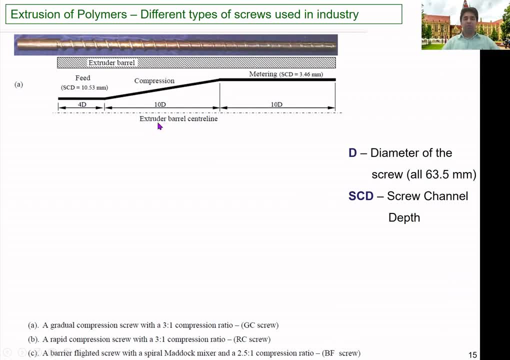 So, if you remember, in the previous videos they were talking about the compression ratio. Okay, So in the compression zone, as I mentioned a while ago. so it has a decrease in channel depth, Okay, Or the channel depth is gradually decreasing, But the channel depth in the peat zone 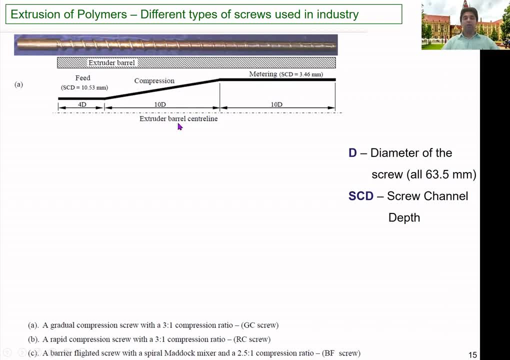 and the metering zone are quite constant. Okay, So the ratio between the peat zone's channel depth and the metering zone channel depth we call is the compression ratio of a screw Right. Sometimes, depending on the some certain conditions like material type, we have to select a screw with the proper compression ratio. 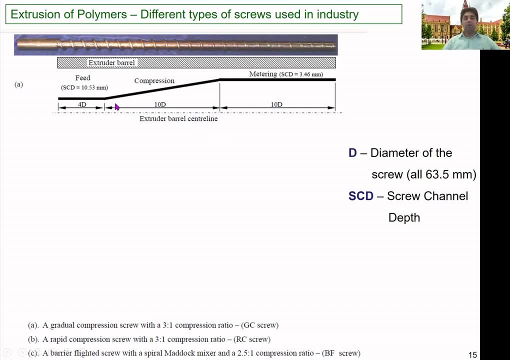 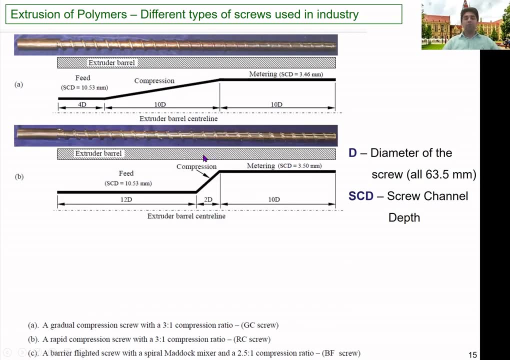 Right, So this is a gradual compression screw, So it is gradually just compressing the material along this length actually. So then the second one we call is the rapid compression screw. So then you could see that. so it is a rapid melting zone, or very quick melting zone. 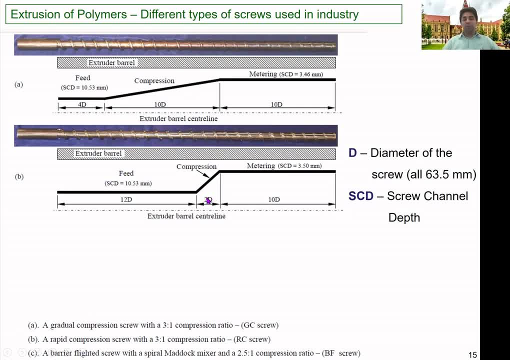 So it has only a length of two diameters of this screw Right. So here also the peat zone. you could see that is 10.53 millimeters, same as this one, And then the metering zone has the 3.5 millimeters should be exactly similar to this. 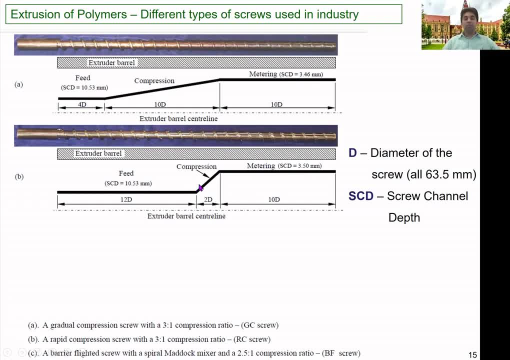 But, okay, the main difference between them two is that the length of the compression or the melting zone, Right The gradual compression and this is a rapid compression, So you can recognize the difference between them Right. So this screw might not be used for some certain material, Okay. 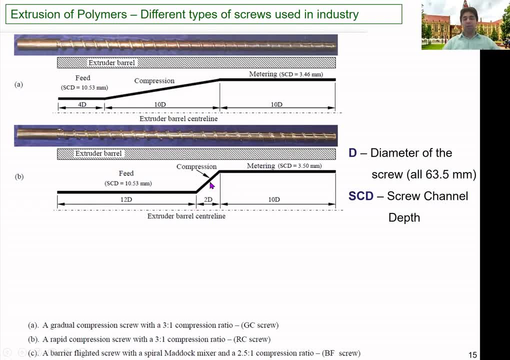 So, because it has a very short decompression zone, So therefore you have to be carefully click this cool, depending on the conditions related to the process. actually, Right, The third one we call it is the barrier plated screw. Okay, it has a different type of the channel arrangement. 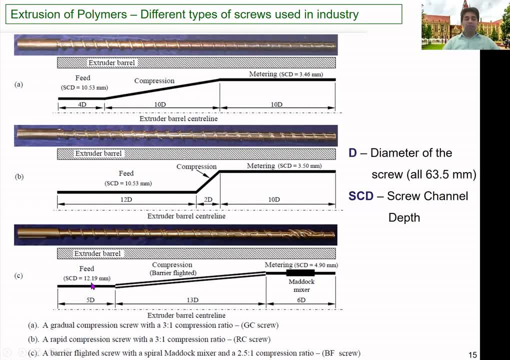 As you can see, here in the peat zone, the channel depth is 12.19 millimeters, here for this one, And then here you can see a special type of arrangement. We called it contact depth, very applied. okay, so you can see it here clearly. so it has a dual channel, okay, so that means that. 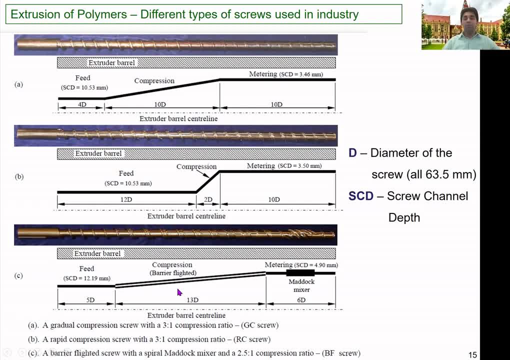 zone or the- this is screw, can get separate the molten material and the unmelted particle into two different channels actually. so that is the idea here, okay. in addition, compared to these two type of screws, it has a mixer at the end, the mixing element. okay, so we call it the maddock. 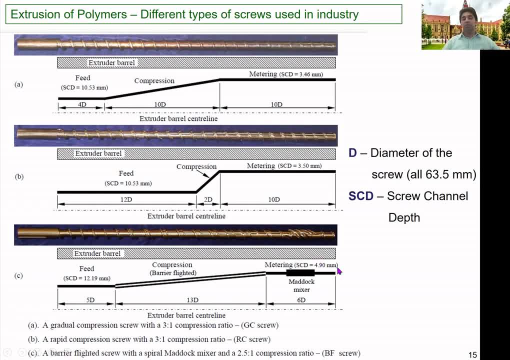 mixer and also the channel depth is in this zone is relatively higher compared to these two. is is greater than maybe 1.4 millimeters compared to these two. it is. it is 4.9 millimeters. the channel depth in the metering zone right and also you could compare the length here: this is five. 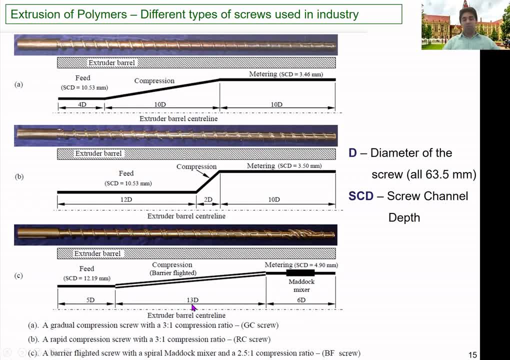 diameters 13d and then 6d. here the longest is the compression zone, so if you want to compare the melting performance of these three screws. so, based on some of my experiments, the, as i discussed some of the results in the last the week in the wednesday morning as well. so the barrier battery. 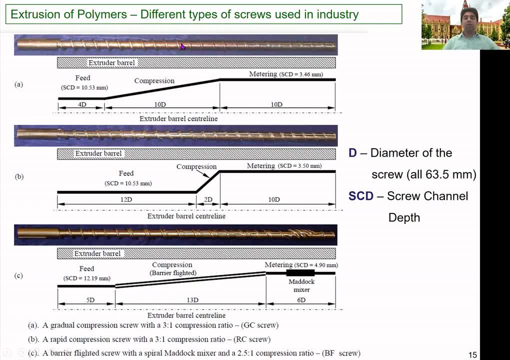 screw is having a better measure of the melting performance of these three screws. so based on some of my experiments in performance compared to this, the gradual compression and rapid compression screws: okay, so you can see that the compression ratios here three to one for the gc screw. so that means 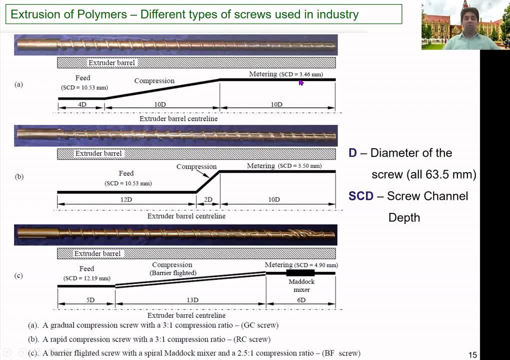 that the 10.53 divided by 3.46, it's just. you could say it is the three to one. the same for the rapid compression is square as well. so here, 12.19 divided by 4.9 will give you 2.5 to one compression ratio. 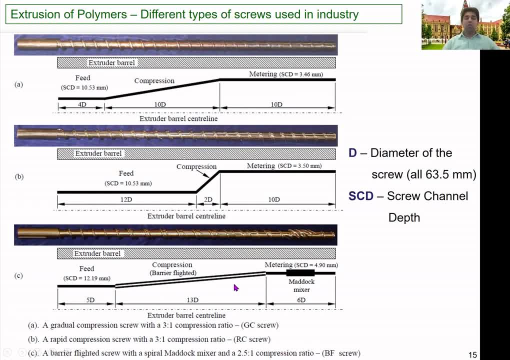 for the barrier plated screw. okay, so these are the common type of screw designs used in industry. if you compare the prices of these screws, actually the barrier plated squeeze is slightly expensive compared to these two. okay, so these are conventional screw design types and these are kind of related. 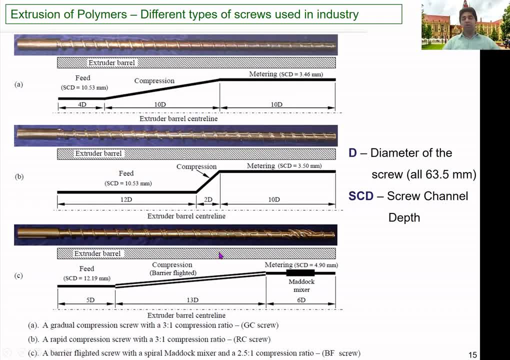 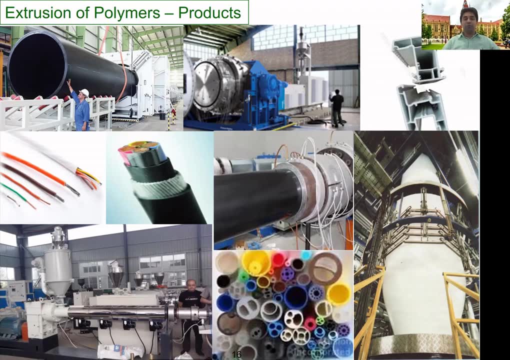 to new school design, and also there are some other new designs recently introduced to the industrial applications as well, depending on the new type of materials and also to improve the melting performance or the conveying performance of the material. in this slide you can see some of the product manufactured using extrusion. okay, you could see how. 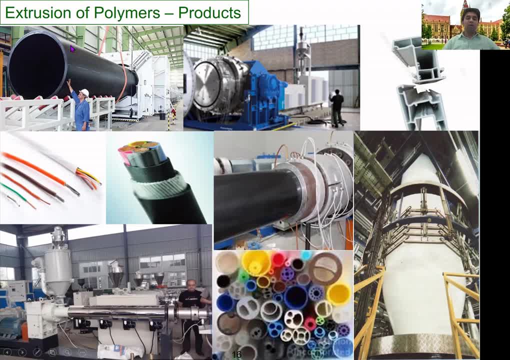 big these machines could be right. okay, so you can see the size of the product. it could be the few meters of diameter and also thickness, could be the five, six centimeters as well. okay, for this scale machine, you have to provide the hundreds of kilograms of material per minute to produce this. 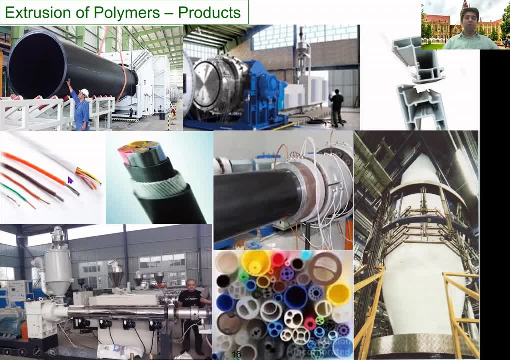 big structure or this big pipe. actually, okay, here you can see some metal wires with coating, and also here you can see multiple wires with coating. again has another common coating, and also this example of another, the electrical wire. so which number of different layers, and then all are being made. 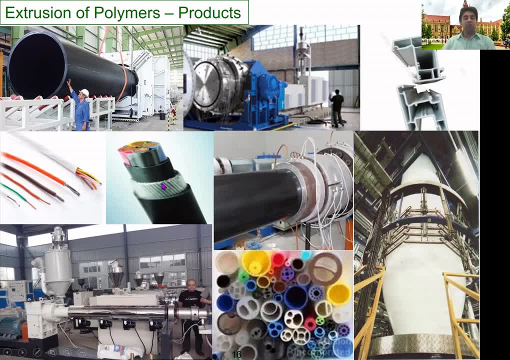 using extrusion. actually, you want to create or manufacture this type of special type of structures. the main element that you have to change is the die of the machine. okay. the rest of the machine is quite the same. only difference is the size. okay, but the main element here. if you want to just 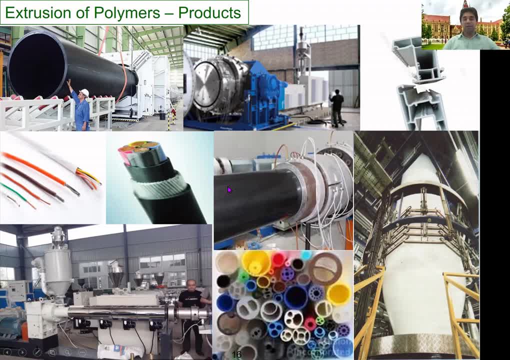 change the design into different formats, is the change in the die? okay, so for example, now here, this is a special type of die to manufacture the pipes. okay, so this is also a small scale pipe coming out from extrusion machine. so here you can see the complete arrangement of extrusion line. so this is the motor that i discussed before and then there. 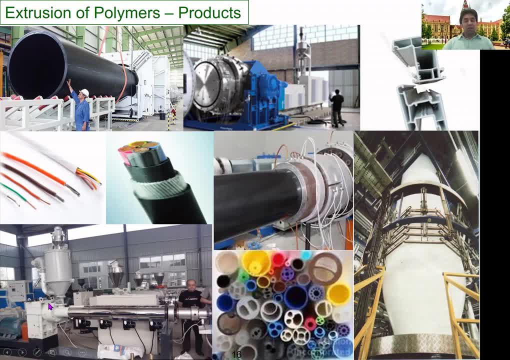 could be a gearbox inside, and then here is connected with the screw inside the barrel and this is the control unit and this is the, the feed hopper. okay, and then here you could see the screw extruder barrel is just the, the wrap, with some sort of insulation to minimize the. 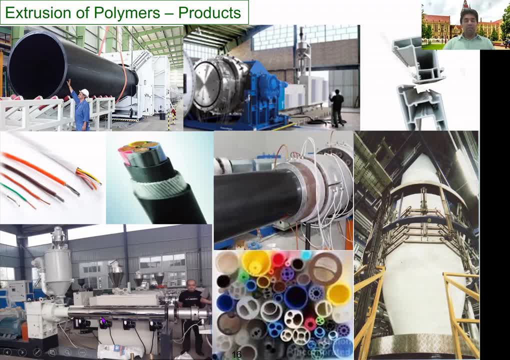 heat loss to the surrounding. and then these are the cooling pads that i mentioned earlier before. so it has four cooling pans and also here you could see the four different temperature zones, uh, the here one, two, three, four, here you can clearly, so you see them. and here there's a clamp ring and 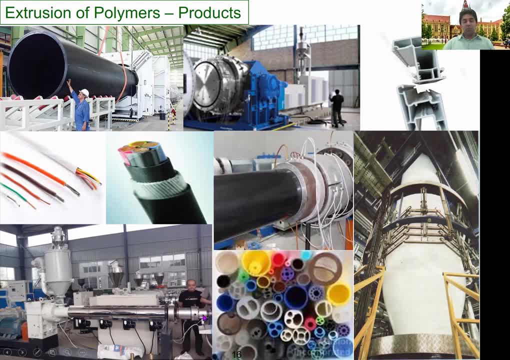 then it has been connected to the die here, okay. so all of these swords should have a different heater to maintain the required temperature, okay. and then there are some other interesting: the cross sections or the arrangements manufactured using extrusion, and also here you can see some kind of the complex. 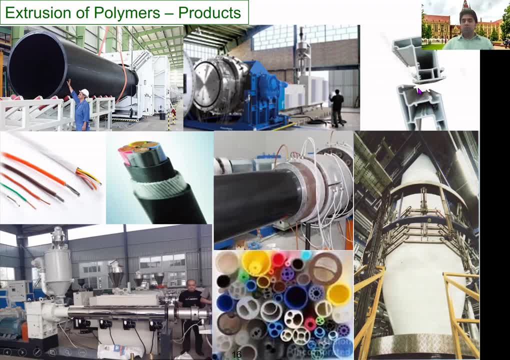 geometries extrude uh through extrusion machines, so this could be even metal as well, so you can use the metal extrusion and also uh the, but it has a different arrangement compared to polymers. so this is what i mentioned before as the blown film extrusion, so which is used to manufacture the thin films. 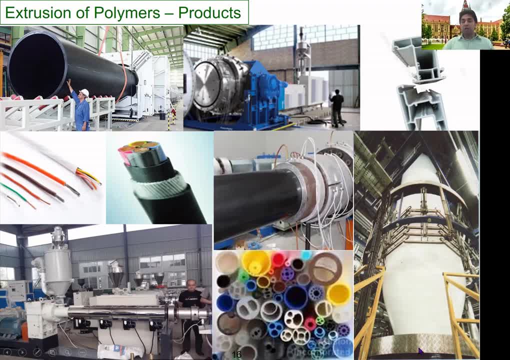 for packaging applications, okay, and here also we have a special type of dye and also we have to use a compressed airline to pressurize the bubble, to to maintain or to control the desired properties of the the film, okay. so this is a good indication of how important extrusion processes and also how important 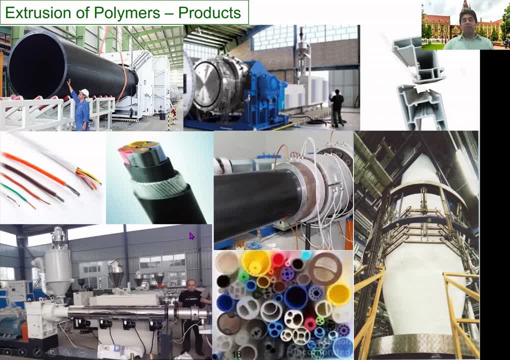 polymeric materials nowadays, so uh, which is being named as the the material of the 21st century right.